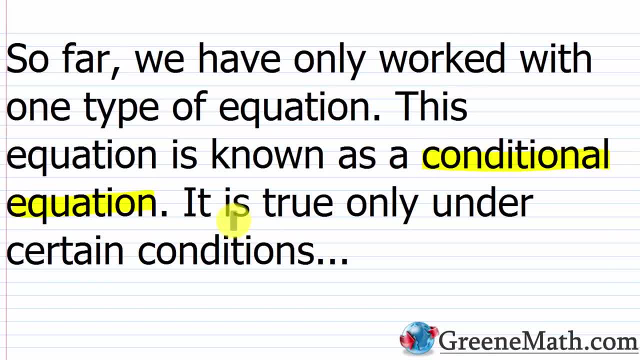 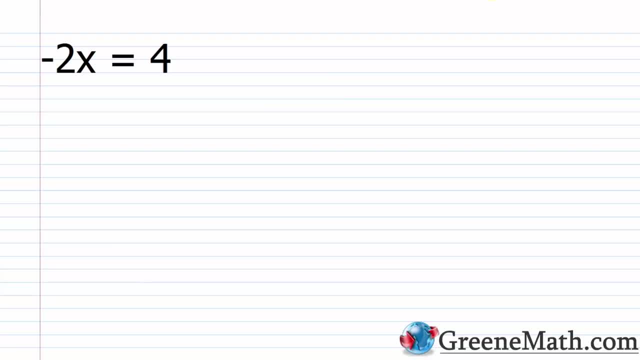 that a conditional equation, So it is true only under certain conditions. So let's see an example. So here's a very simple example of a conditional equation. Everything we've worked with so far has been a conditional equation. So negative 2x equals 4.. So we all know how to solve this at this point. 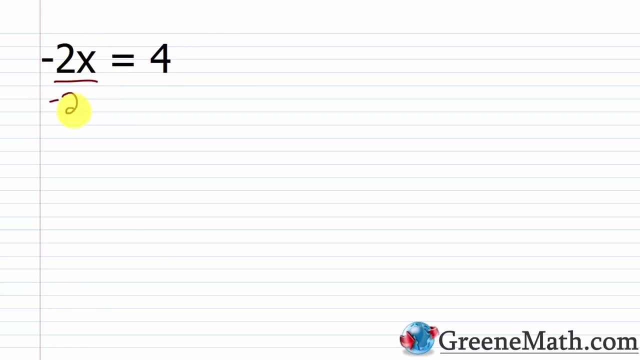 Right, we want to isolate x, So we divide both sides of the equation by negative 2. Right, the coefficient of x This cancels with this and becomes 1.. So I have: x equals 4 divided by negative. 2 is negative 2.. So that's my solution. Now, the reason it's called a conditional equation is because 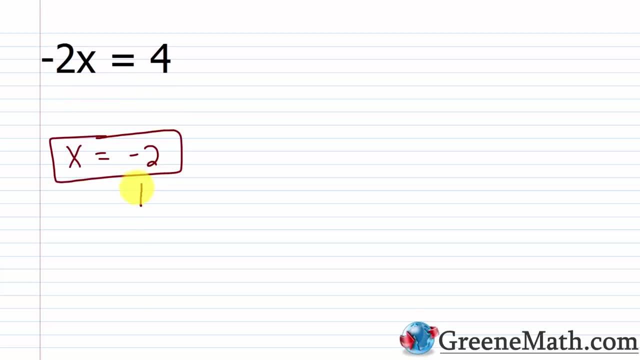 this equation is true under this specific condition That x is equal to negative 2.. If I plug in a negative 2 for x, I would have negative 2 times negative. 2 equals 4.. And then this left side simplifies to 4.. So 4 equals 4.. So that all checks out Now. 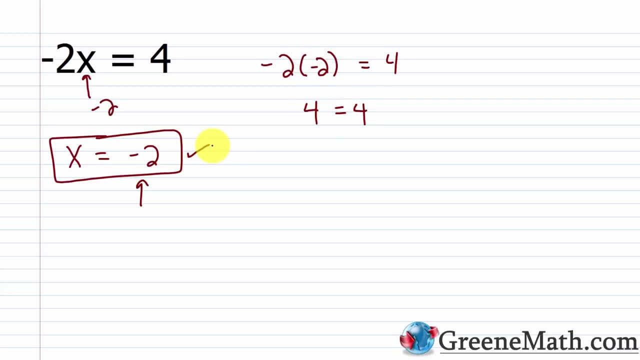 if I choose anything else for x. this is no longer a true statement. If I was to say, if I was to say, x is equal to negative 2. If x is equal to 7, for example, Well, negative 2 times 7 is not equal to 4.. Negative 2 times 7 is: 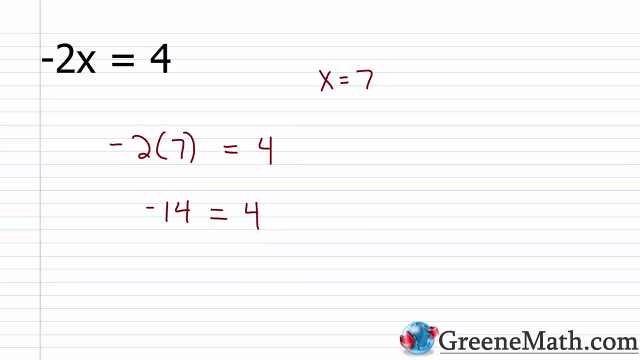 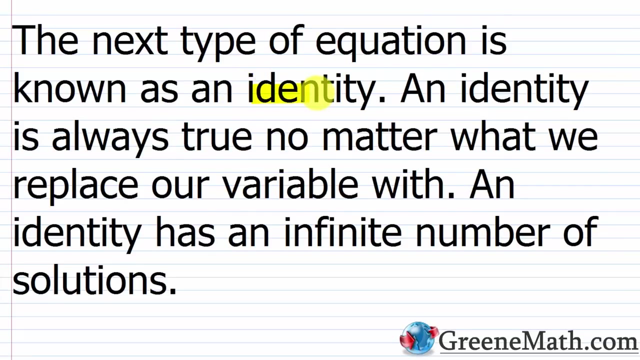 negative 14.. That's not equal to 4.. This is wrong, Wrong. Okay, only if I use x equals negative 2 will this equation be true. All right, so the next type of equation is known as an identity. Okay, an identity. An identity is always true. Okay, no matter what. 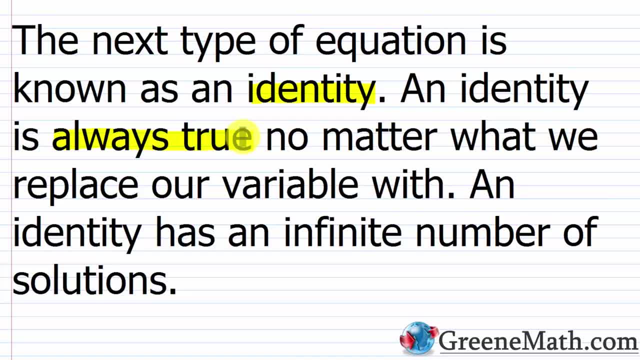 What we replace our variable with. So we can replace it with a billion negative 2,, 4,, 27,. negative 1. fourth, It does not matter, It will always be true. The key thing is that an identity has an infinite number of solutions. So here's an example of an identity. So we have 3x minus 12. 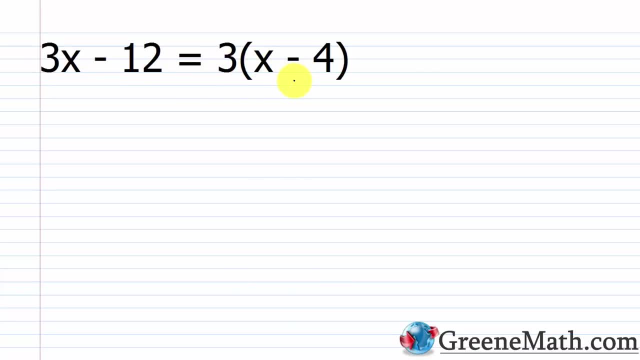 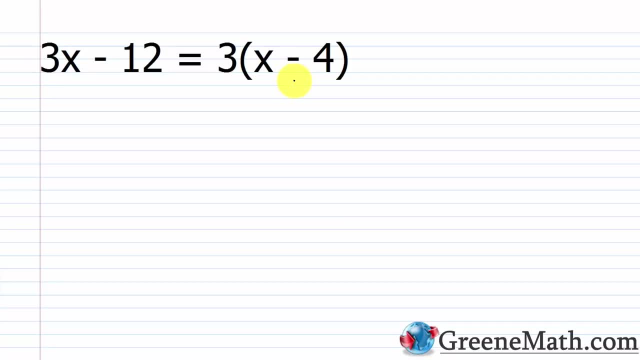 pick any number you want, Doesn't matter what it is, And plug it in for x, and I bet it works. I'm going to pick the number I don't know, negative 8.. So I'm going to plug in a negative 8 here and 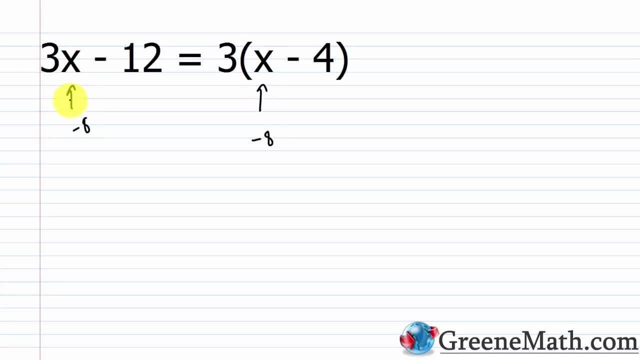 a negative 8 here And let's see if we get a true statement. So 3 times negative 8 is negative. 24 minus 12 equals 3 times the quantity negative 8 minus 4.. So negative 8 minus 4.. And negative 8. 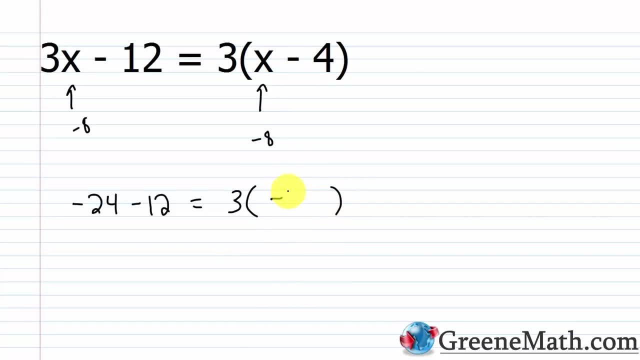 minus 4 is negative 12.. I would have 3 times negative 12 on the right, So this is negative 36.. Over here, negative 24 minus 12 is negative 36 also. And you might say, okay, well, you solved that already. You knew that x was equal. 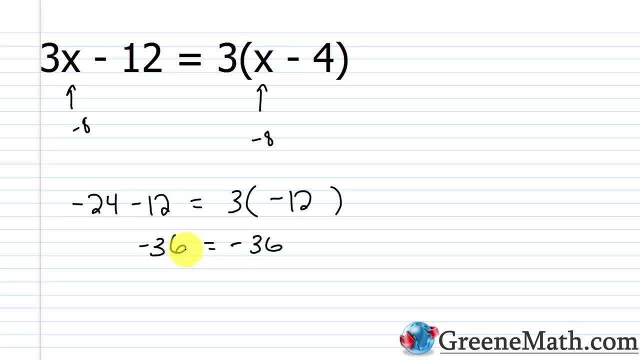 to negative 8. Pick anything else. Let's pick 4, for example. Let's pick 4 and see what happens. So I'll plug in a 4 here and I'll plug in a 4 here. So 3 times 4 is 12 over here minus 12.. We'll. 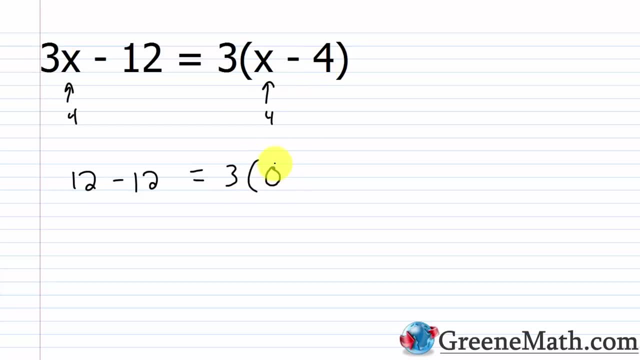 over here I'll have 3 times the quantity 4 minus 4, which is 0.. So 3 times 0 is 0.. Over here, 12 minus 12 is 0.. 0 equals 0. So that's a true statement. Let's try one more. So now, let's try. I don't know. 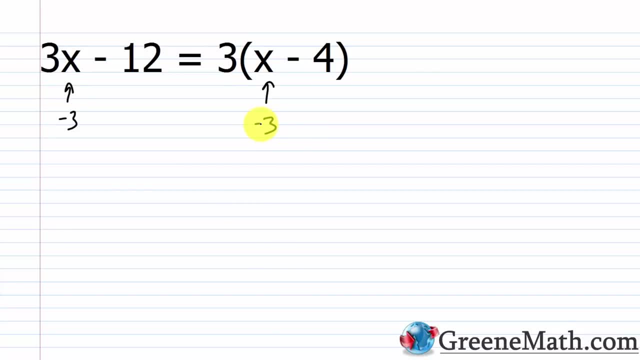 negative, 3. Negative, 3. So 3 times negative: 3 minus 12 is equal to 3 times the quantity negative 3 minus 4.. So over here: 3 times negative, 3 is negative, 9.. Negative: 9 minus 12 is negative 9.. 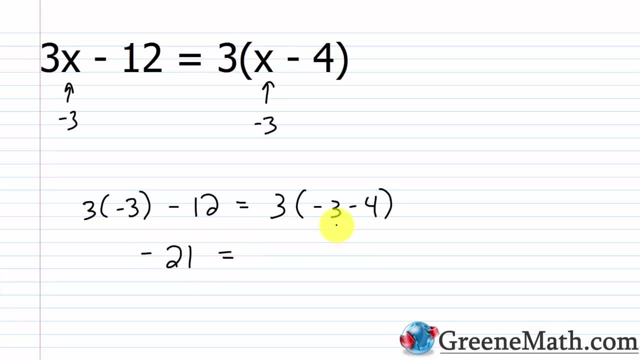 Negative 9 minus 12 is negative 21.. Over here, negative 3 minus 4 is negative 7.. 3 times negative 7 is negative 21.. So again, again, again. I get: the left and the right side is the same value. So how can? 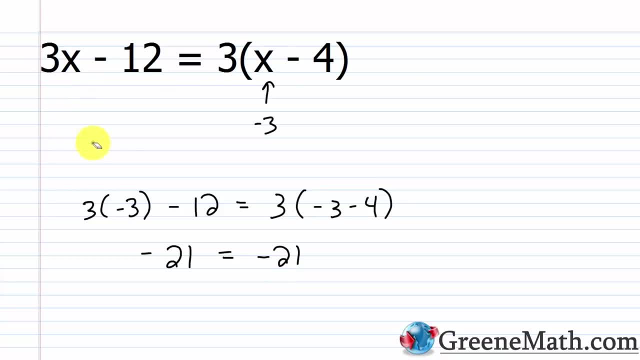 that be the case. Well, the trick to this identity is, if you haven't noticed it already, the left and the right side are the exact same thing. They're just in different forms. This over here is just a simplified version of this over here, If I use my distributive property, 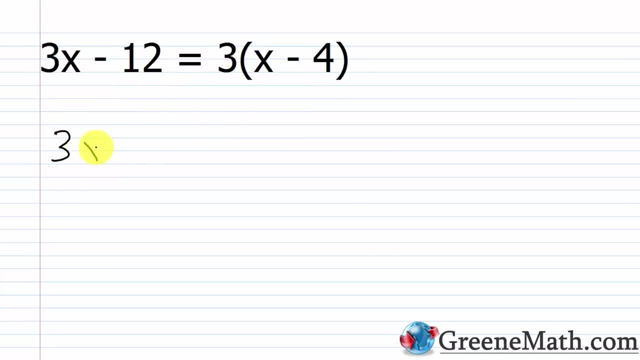 on the right side, so the left would still be 3x minus 12.. 3 times x is 3x, and then minus 3 times 4, that's 12.. So I have the exact same thing on both sides of the equation. So, of course, 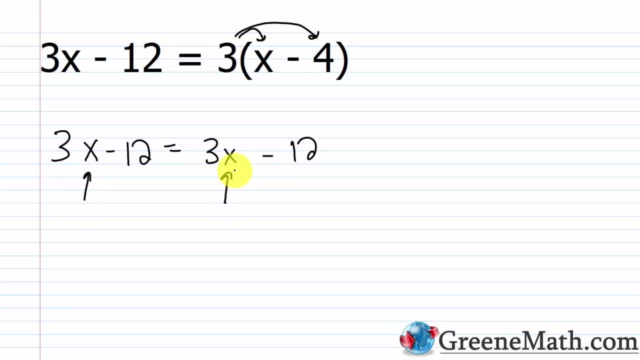 whatever I plug in here and here, I'm going to get the same value, because I'm doing the exact same thing. If I plug in a 2 here and I plug in a 2 here, in each case I'm multiplying 3 by 2 and 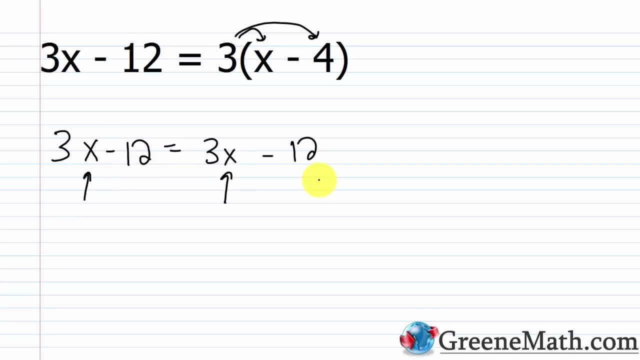 then I'm subtracting away 12 on both sides, So it doesn't matter what number I'm going to get, I'm I do the exact same thing to it, and so the left and the right side will always be equal. and so there's an infinite number of solutions, because I can choose any number that I want, right It's. 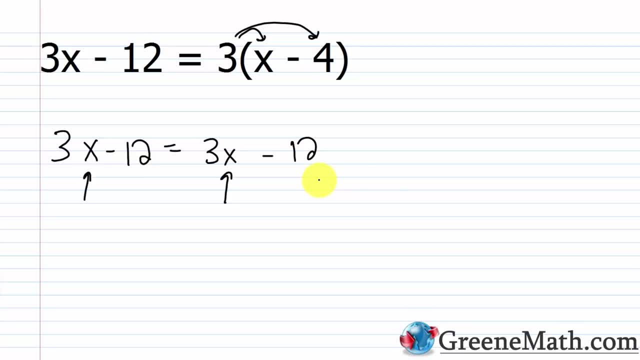 literally unlimited as far as how many solutions you would have. So if you were to come across this in your textbook, or your teacher gives it to you for homework or a test, just write that the solution is all real numbers. And as we move throughout algebra we're going to see some. 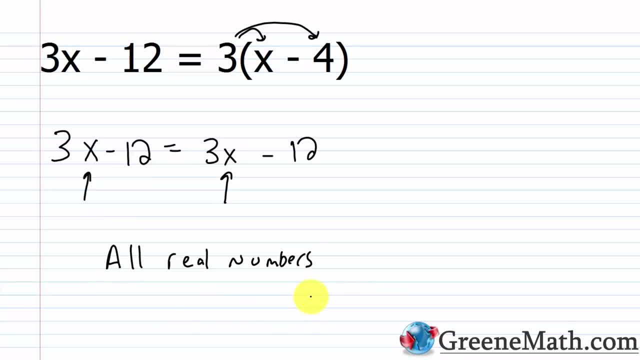 different notations that we're going to see. So let's say that we're going to see a number that we're going to use to say, hey, all real numbers. Right now, we're just going to write it out. Okay, we're not ready for the notation yet, So we're just going to write all real numbers. That's your. 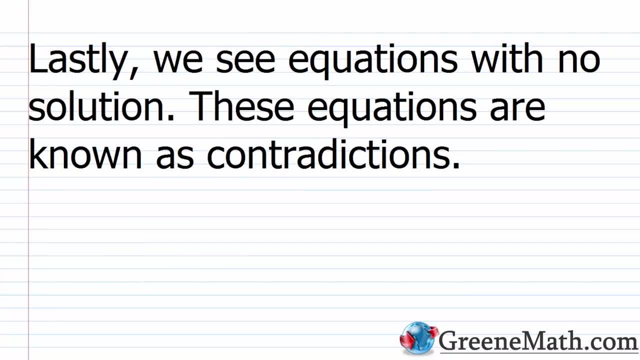 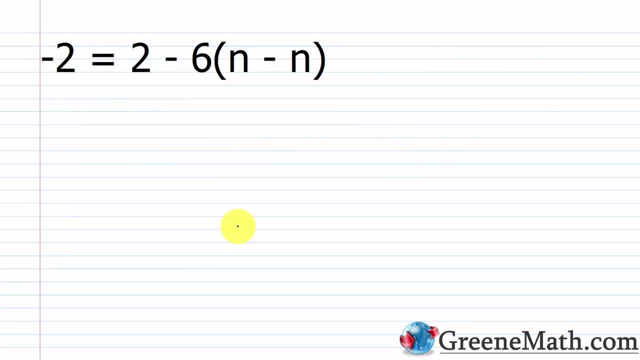 solution, All right. so, lastly, we see equations with no solution. These equations are known as contradictions. So contradictions. So no matter what you choose for n, it's never going to work. And to see why, let's? let's simplify the right hand side of the equation. So negative 2 equals. 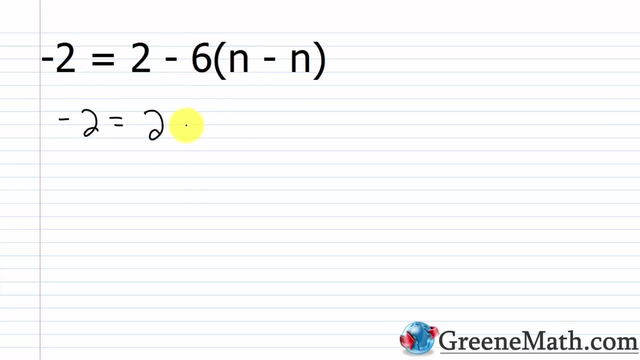 we have 2.. We have negative 6 times n, That's negative 6n. Then we have negative 6 times negative n, That's positive 6n. So what you're going to see is that, if I simplify the right hand side here, 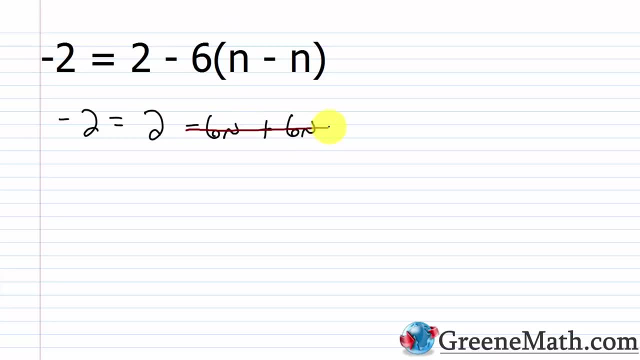 the variable n is going to go away. completely. Negative 6n plus 6n- those are opposites. Those are gone. So what I'm left with is just nonsensical statement that negative 2 equals 2.. Well, it doesn't. This is wrong. Negative 2 doesn't equal 2.. So nothing is n, It's just a. 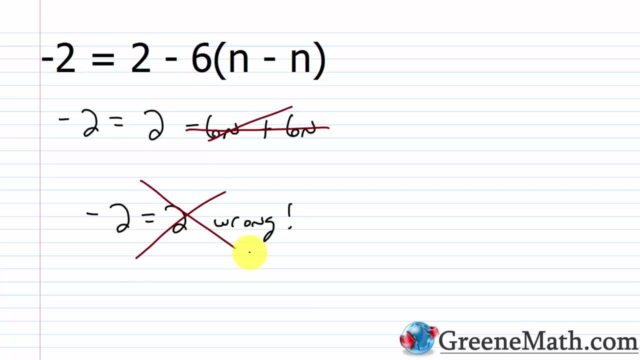 nonsensical statement. So what you're going to see is that if I put something in for n, I'm just going to subtract it away. So the result of this would be 0.. Right, I plug something in for n, I subtract that same number away. I get 0.. I multiply 6 times 0.. I get 0.. So I'm just left with. 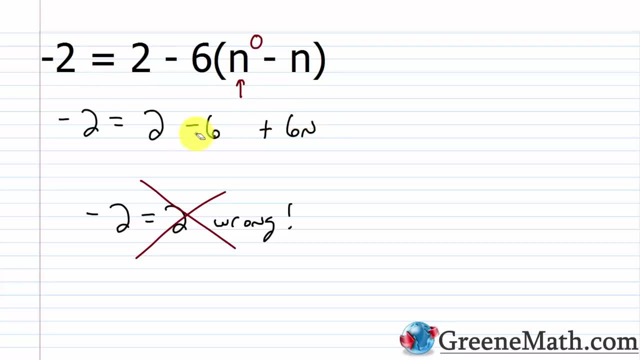 negative 2 equals 2.. Right, Once I simplify, This is what I'm going to have, no matter what I choose for n Negative 2 equals 2.. So there's no value of n. It can ever be chosen. that will make this a true statement, And so this is an example of a 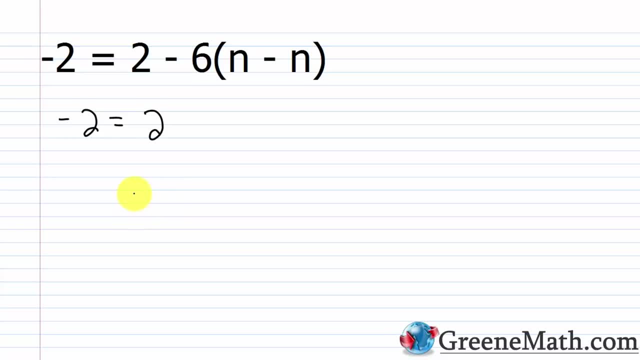 contradiction And so when this occurs, you can put no solution And again we'll have some fancy notation for that moving forward, But for right now just put no solution. Hey, there's, there's nothing I can do here. So let's look at some examples and let's see if we can figure out. 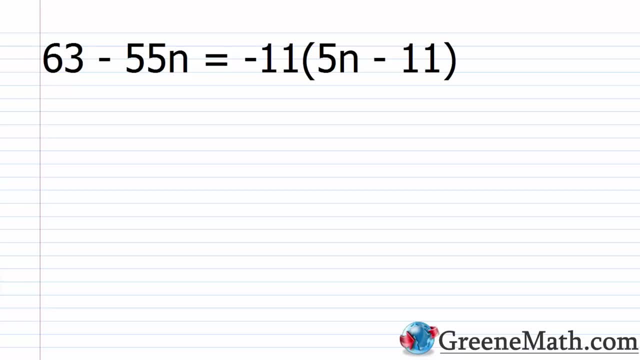 through simplification what type of equation they are. So this one I have: 63 minus 55 n Equals negative 11 times this quantity, 5 n minus 11.. So on the left, 63 minus 55 n. On the right, I'm going to use my distributive property to remove the parentheses. So negative 11 times 5 n. 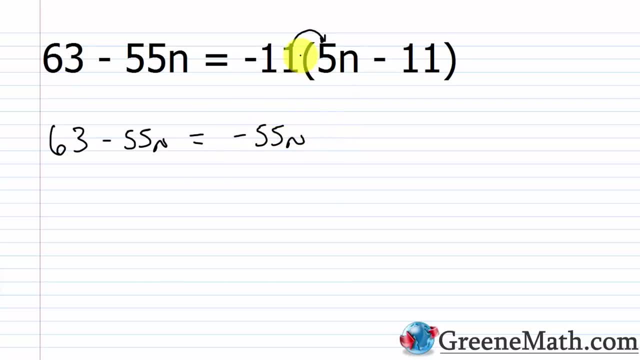 That's negative 55 n. And then I'll have negative 11 times negative 11.. That's positive 121.. I told you this in one of the videos I made in a previous lesson or practice, I can't remember which one. If you have the exact same number on two sides of the equation, 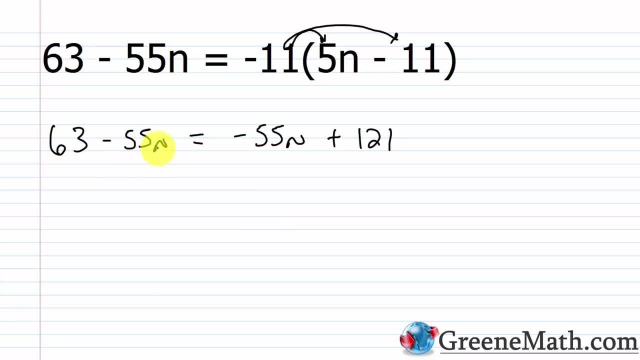 you can get rid of it. In other words, I have negative 55 n here, I have negative 55 n here, I can just get rid of it. Why is that the case? Well, through the addition property of equality, I can legally make it disappear. If I add 55 n here and I add 55 n here, I've added the same. 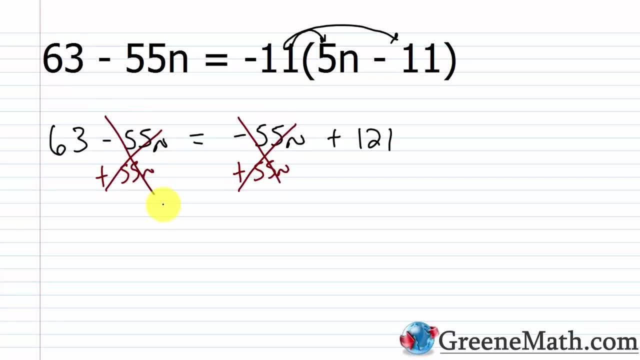 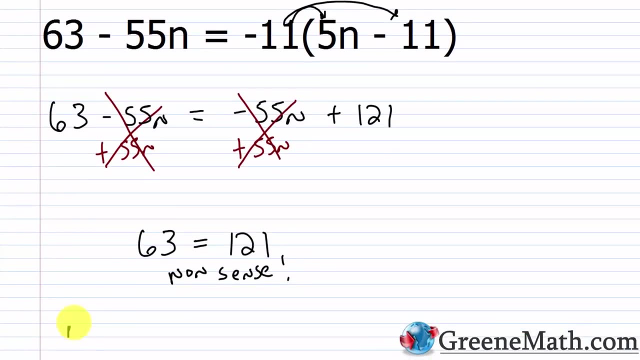 number to both sides of the equation. In both cases it's gone, It sums to zero And I'm left with 63 equals 121. Which again is nonsense. This is nonsense. Okay, in case you don't know. So there's no solution here. No solution. This is another. 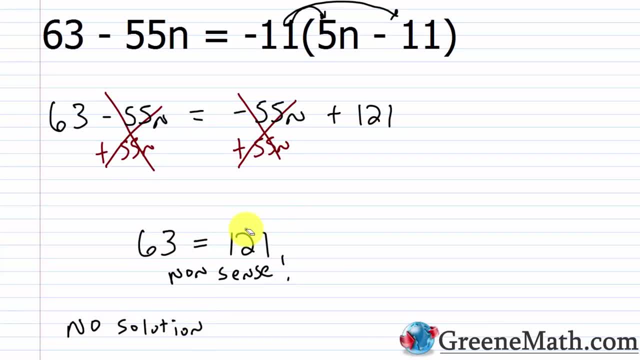 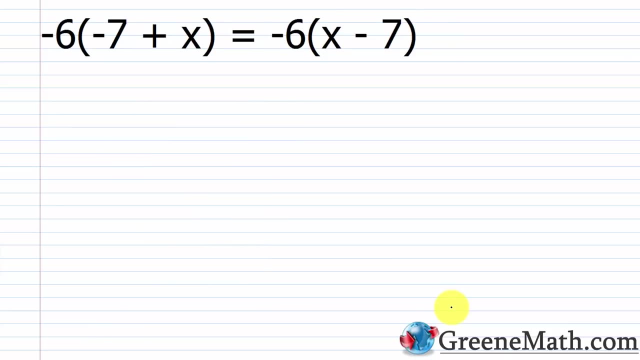 example of a contradiction. All right, if you end up with your variable disappearing and you get you know one side doesn't equal the other, You have a contradiction. There's not a solution, All right, so this is nonsense. All right, let's take a look at this one. We have negative 6 times the quantity negative 7 plus x. 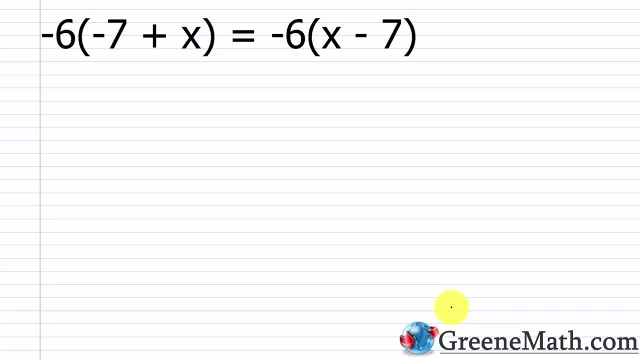 is equal to negative 6 times the quantity x minus 7.. So again, let's simplify: Negative 6 times negative 7 is 42.. Negative 6 times x is negative 6x. So minus 6x Over here. negative 6 times x is: 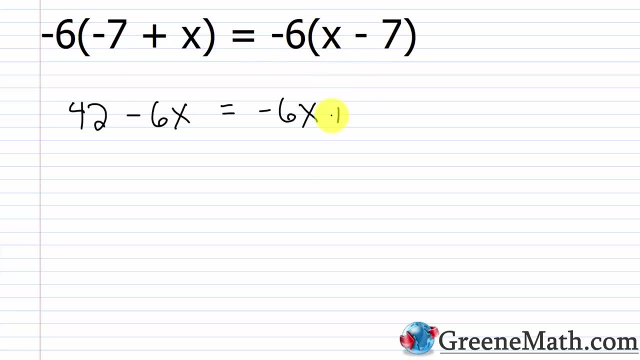 negative 6x Over here. negative 6 times negative, 7 is plus 42. Now, if I look closely, I can see that these are the same Right, this is an identity, And so upon first glance- and I'm looking at this equation up here- 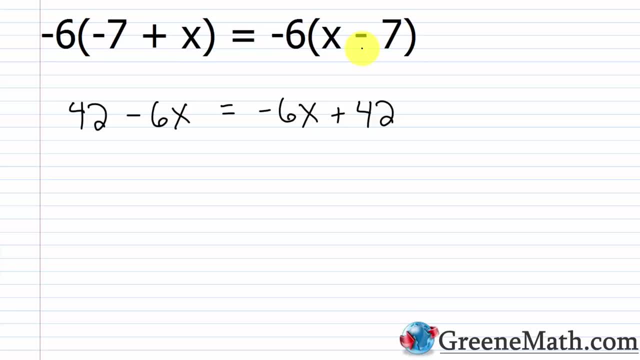 it looks like a regular equation, But once you simplify it and kind of really pay attention, I can reorder this to negative 6x plus 42. And it's the exact same thing as over here: Negative 6x plus 42. So whatever value I choose for x, doesn't matter what it is. I plug it in, I multiply. 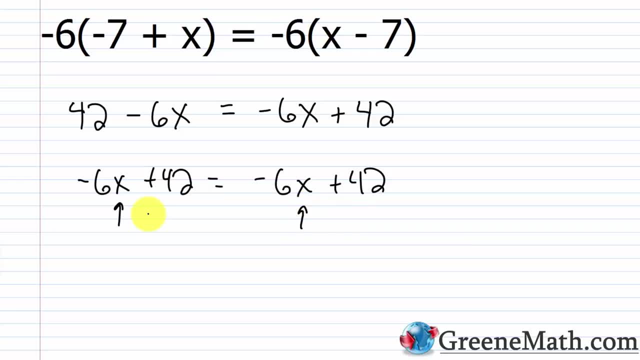 by negative 6 and I add 42 to it. The same thing is going to happen on both sides of the equation, And so I can pick whatever I want for x and it'll be a solution. So this would be all real numbers. Again, this is an identity. All right, let's take a look at another. We have negative 4. 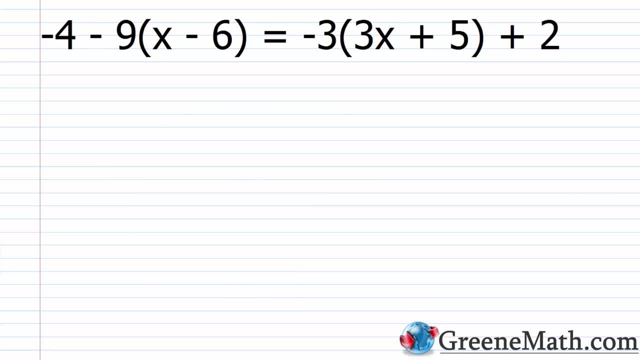 minus 9 times the quantity x minus 6. This is equal to negative 3 times the quantity 3x plus 5 and then plus 2.. Again, I'm going to simplify each side of the equation. I'm going to look to see. 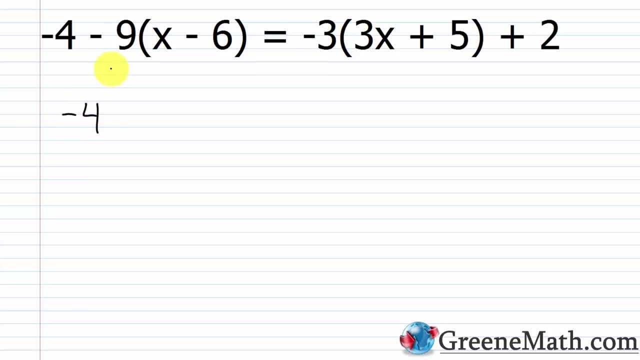 what type of equation I have. So negative 4x plus 42.. I'm going to look to see what type of equation I have. I have negative 9 times x. That's negative 9x or minus 9x. Negative 9 times negative: 6 is plus 54. 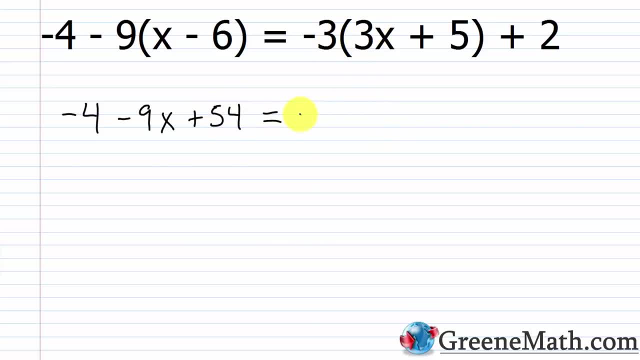 This is equal to: Here: I have negative 3 times 3x, That's negative 9x. Then I have negative 3 times 5.. That's minus 15 and then plus 2.. Now, again, again, again. I've told you that if you have. 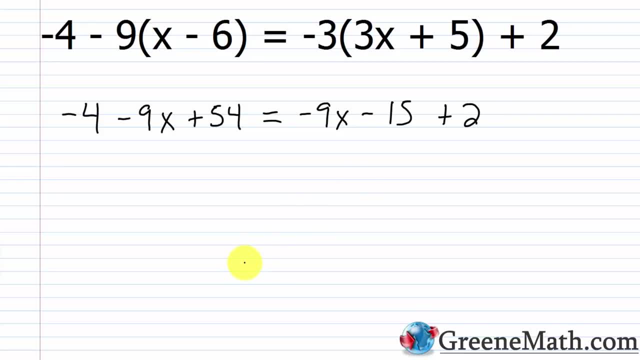